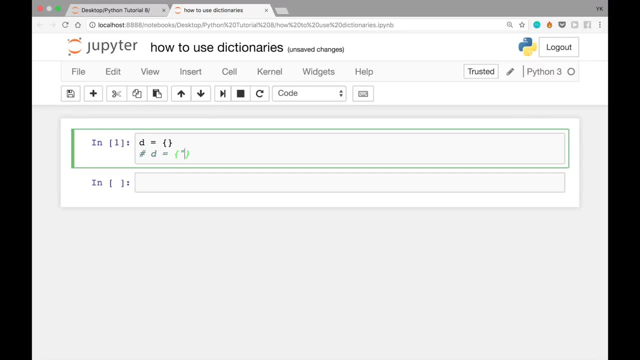 d equals curly brackets. double quotes George, colon 24, comma. double quotes Tom, colon 32.. And this defines a new dictionary with the value 24.. That's associated with the key George and the value 32. that's associated with the key Tom. But let's go with the first one for now to define an empty dictionary. After defining an empty dictionary, you can add a key value pair like, so These: 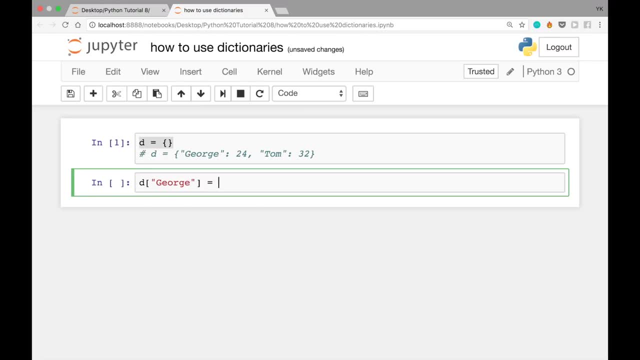 are brackets double quotes: george equals 24. this says: add a new key value pair where the key is george and the value is 24. we can add more pairs by writing: for example: d square brackets double quotes: tom equals 32 and d square brackets jenny equals 16. and now this dictionary has: 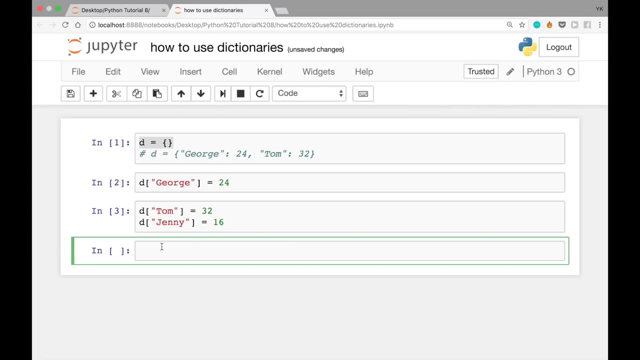 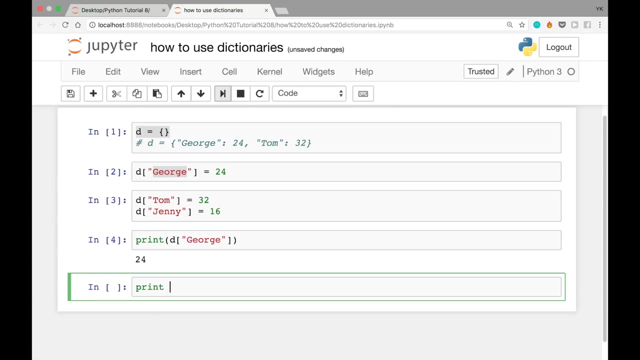 the three key value pairs and to find a value that's associated with a certain key, for example george, you can just write: print d square brackets, george, and this will print out the value that's associated with the value george. and then, of course, if you want to print out the value that's 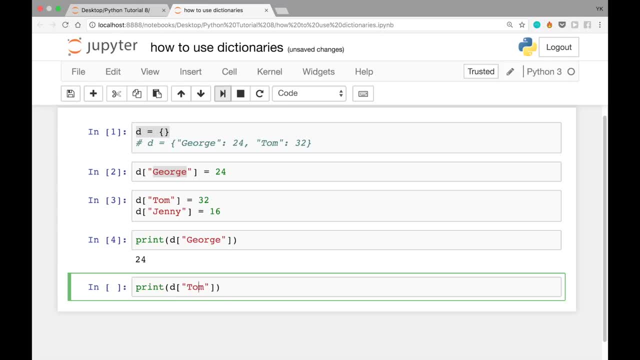 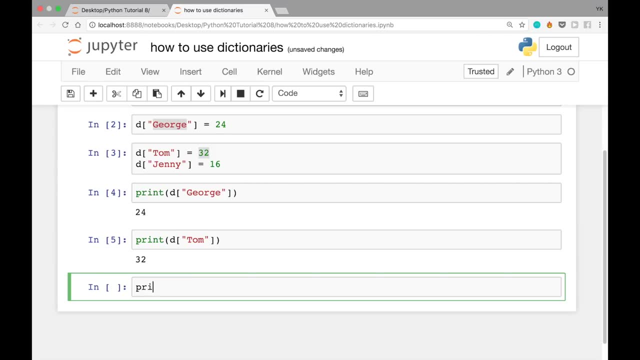 associated with the key tom. you can just write: print d square brackets- tom and then it'll print out 32, and if you try to look up a key that doesn't exist yet, it's going to give us an error. for example, if you do d square brackets. 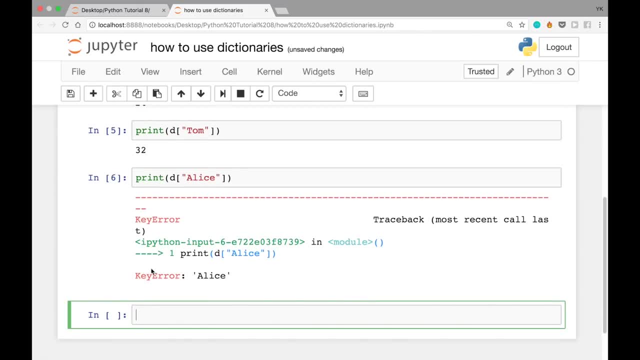 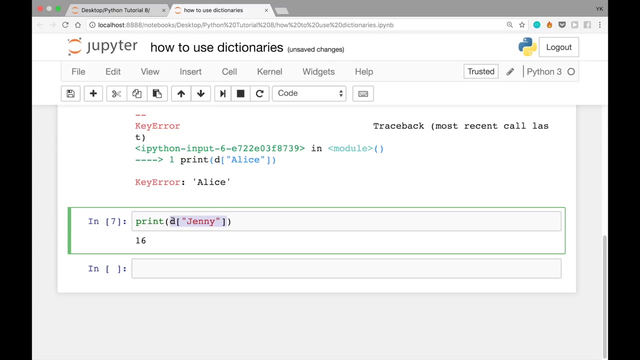 alice. it gives us this key error because the key alice doesn't exist yet. now, as we saw, the value that's associated with jenny was 16. but it's possible to change the value that's associated with a certain key after we already have that key value pair in the dictionary. we can do that with. 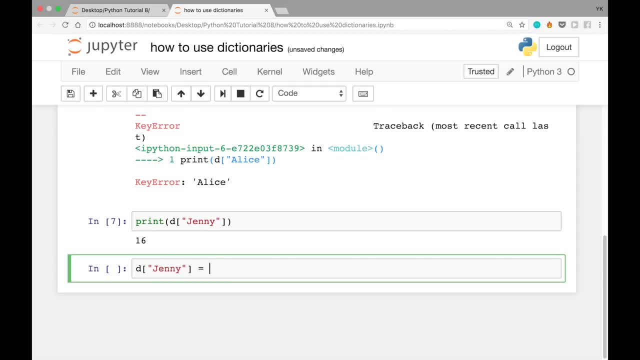 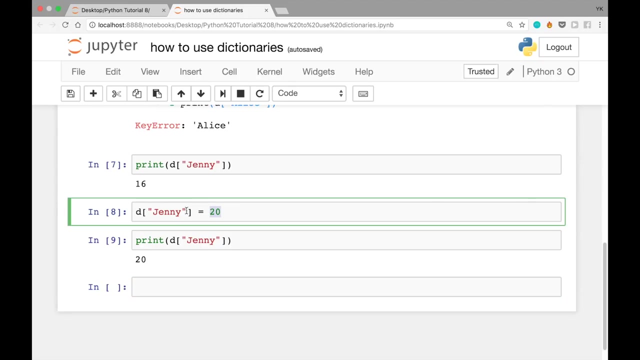 just like before the square brackets, Jenny equals 20, and once we run the cell now, the value that's associated with Jenny is 20. now, one thing to note here is that the values can be any type, but the keys can only be certain types, and there are. 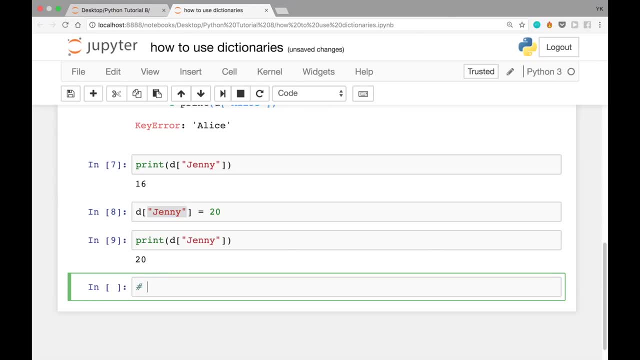 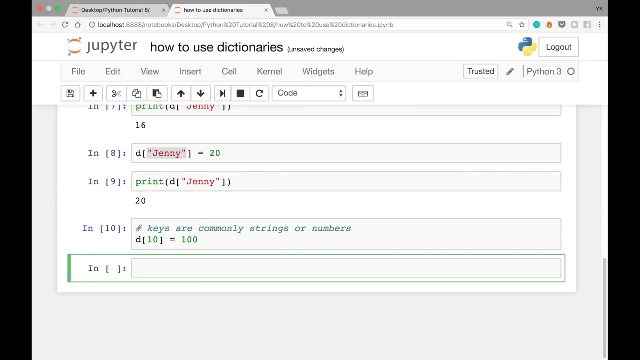 different types we can use for that, but most commonly keys are strings or numbers, and in Python you can even mix different types of keys. so, for example, you can add a new key, let's say 10, with the value 100, to this dictionary D. with D square brackets, 10 equals 100 and once we write print parentheses D square. 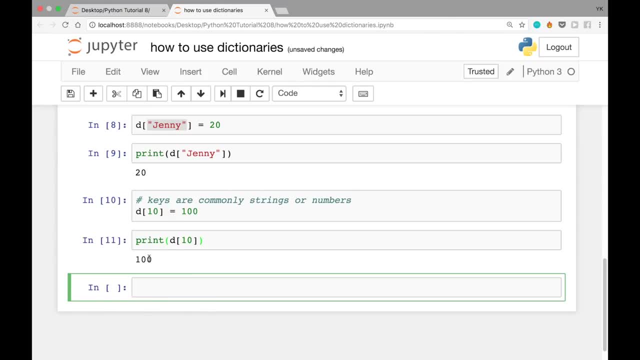 brackets 10, it works just fine. retrieving the value 100. now what if we wanted to iterate over key value pairs in the given dictionary, for example this one D? let's pretend for a second that we don't know how to do that. and of course, if we don't know how to do, 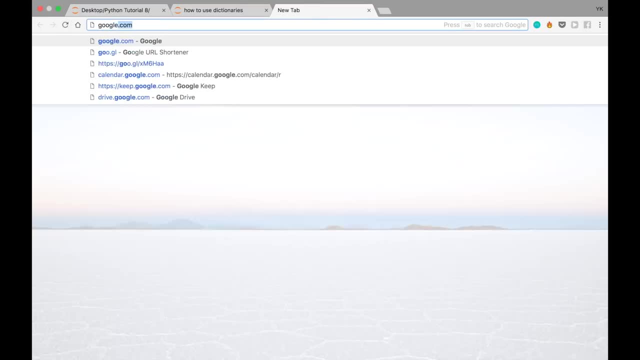 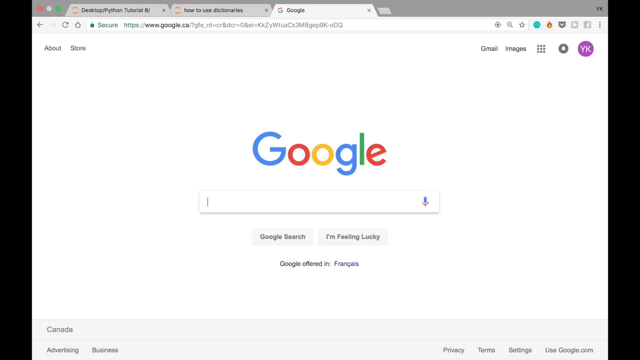 something like that. the first thing we should do is we should just use Google- and I'm going to show you how I would go about it, and for that I might write something like how to iterate over key value pairs, dictionary Python. let's take a look at the first. 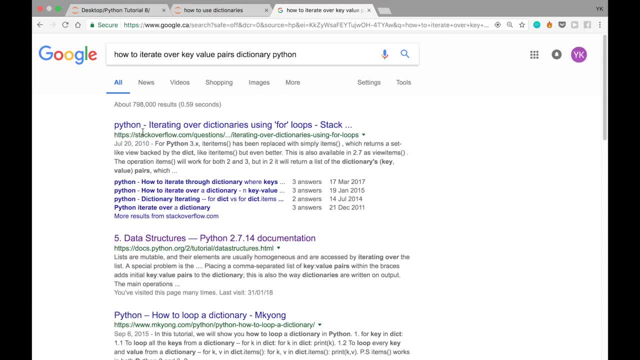 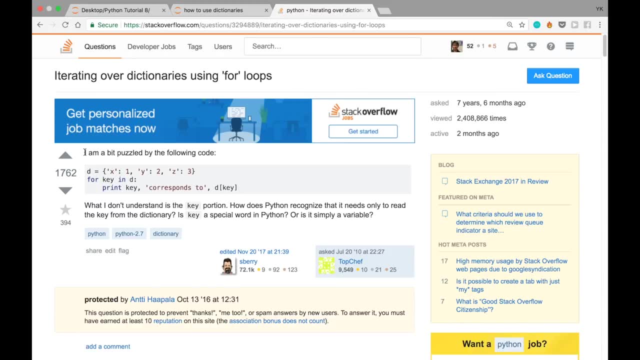 we're going to do. is we're going to do, is we're going to do, is we're going to do. result this one right here from stack overflow, and just be careful because this one is a little bit old- it's from 2010, but it might be okay and you can see. 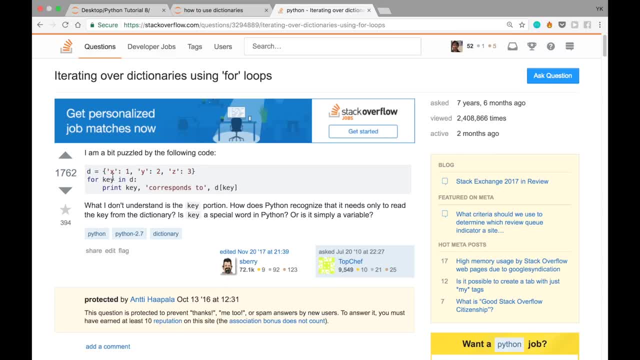 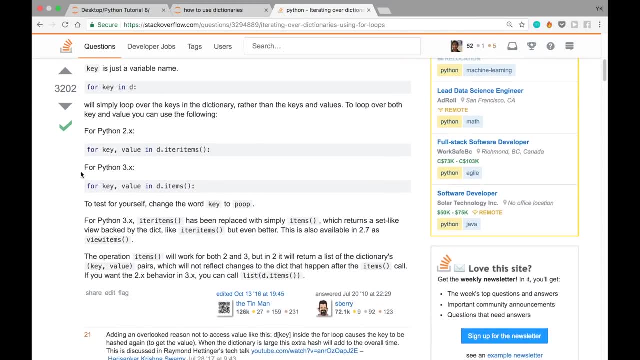 that this question is about a dictionary and then a for loop here, so I would just skim through this page and then I would try to find what I'm looking for, which is something about Python 3 probably. so it says: for Python 3, points X, we're. 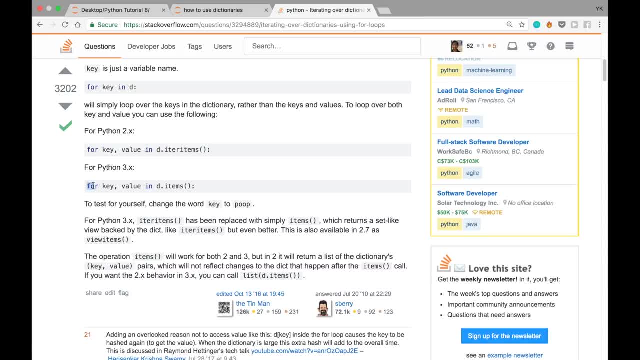 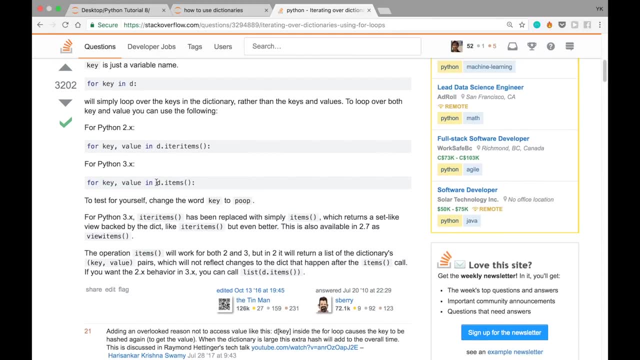 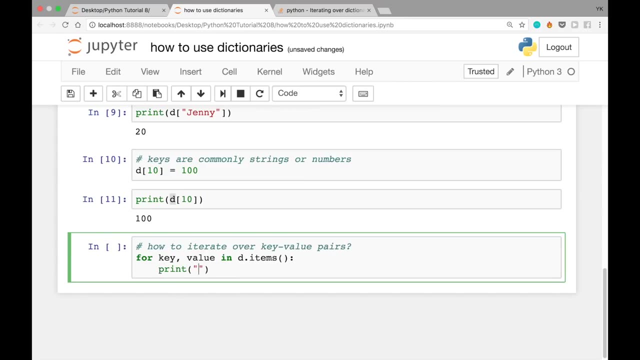 using Python 3. by the way, it looks like we might be able to use for key comma value in D dot items and it looks like this D is the dictionary, so let's see if it works by copying this over here and let's try print key and then key without the double quotes, and then 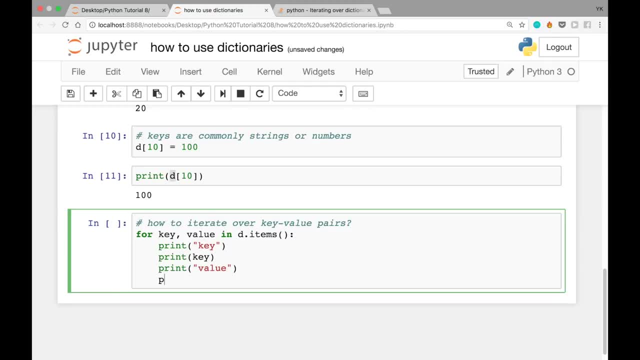 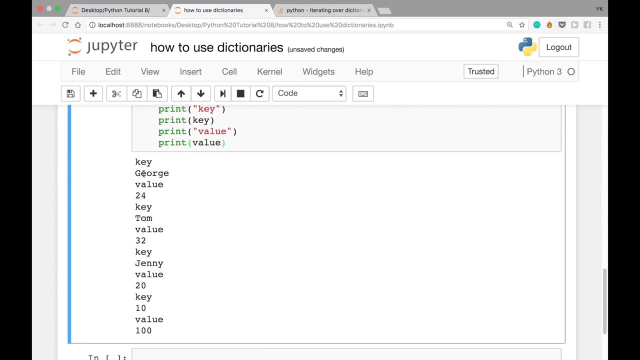 the same thing with the value. so print value and then value, and once we run this cell we see key is the dictionary and then value is the dictionary and then target here so we could validate that we're going to give it a keygorge and then the value that's associated with it is 24 and to make this look a little,